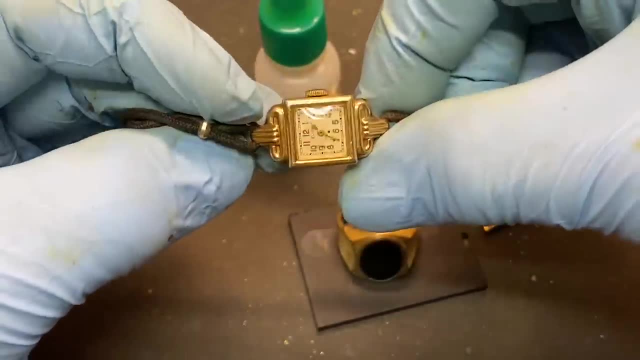 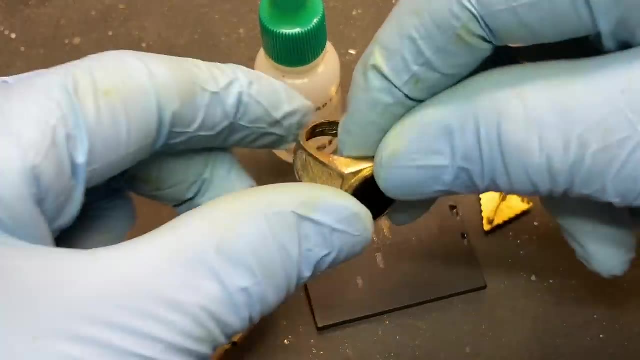 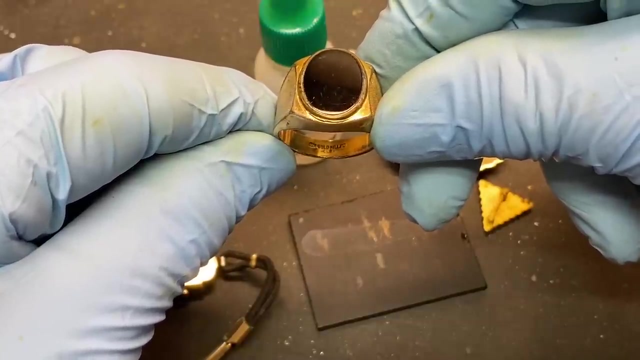 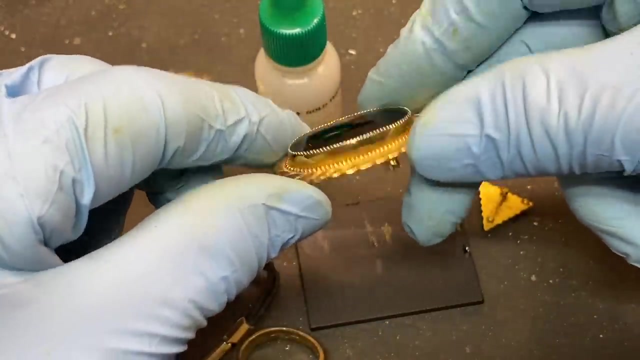 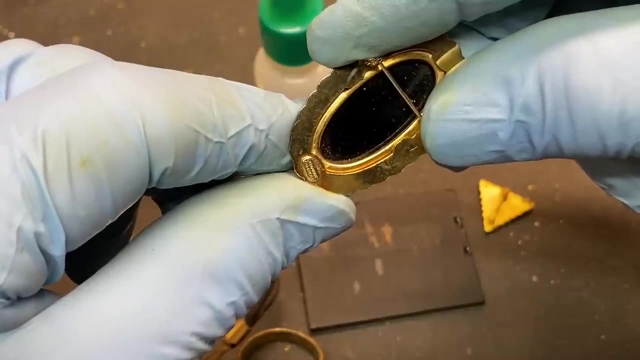 examples of the markings. This is a watch: 14k gold-filled. right on the back there This is a ring and inside there it says 10k gold-filled. I've also got a pendant here, a pin, and down on the bottom down here it says 1, 20th, 12k gf. That's a marking for gold-filled. 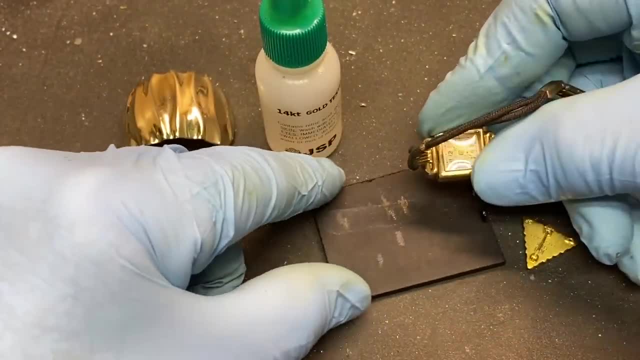 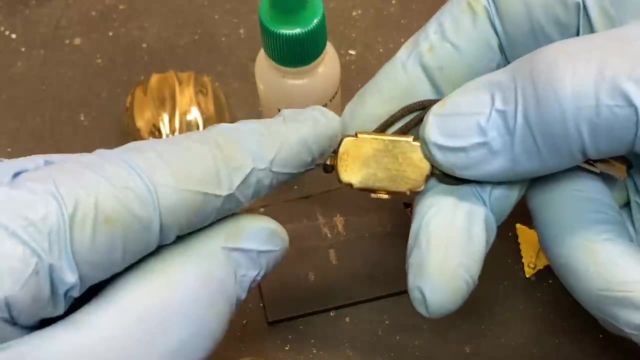 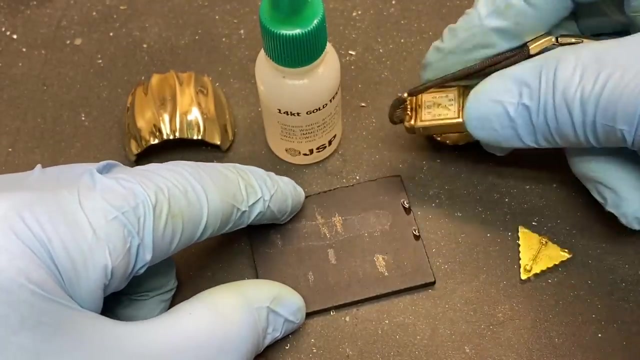 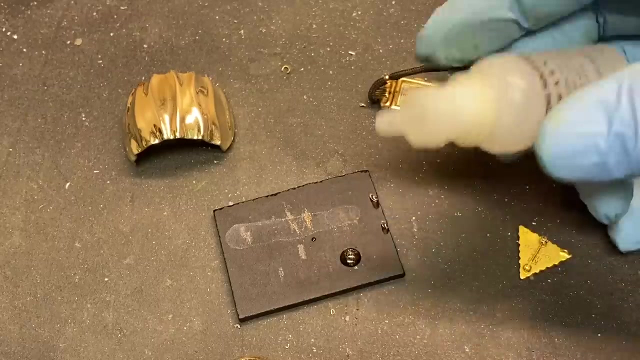 Not all gold-filled pieces are marked. Most usually are, And what I'm going to do now is I'm going to rub some of the gold-filled material on this 14k gold-filled watch onto my touchstone here And we're going to add a drop of acid to it And you'll notice that the test is positive for parrot. 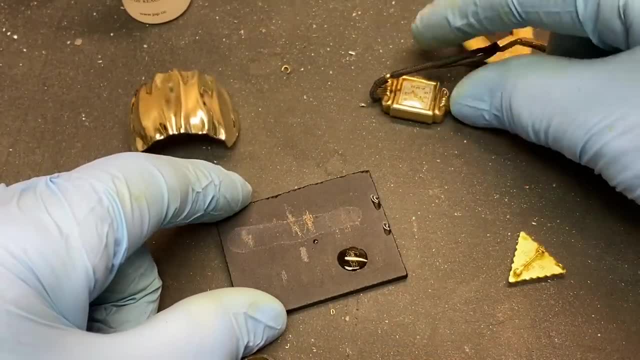 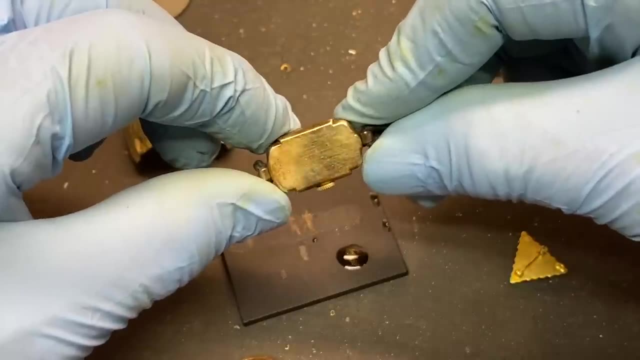 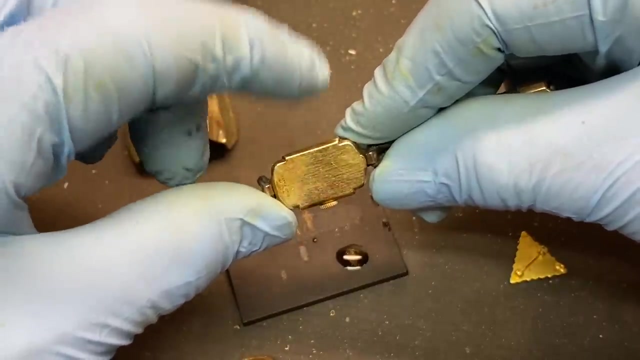 dissolve away. That could be a bad deal for someone testing their carrot scrap for refining, For example, if you have a piece of gold-filled material with a thick coating of gold over brass, like this is, and it tests positive for carrot gold, like this test shows. 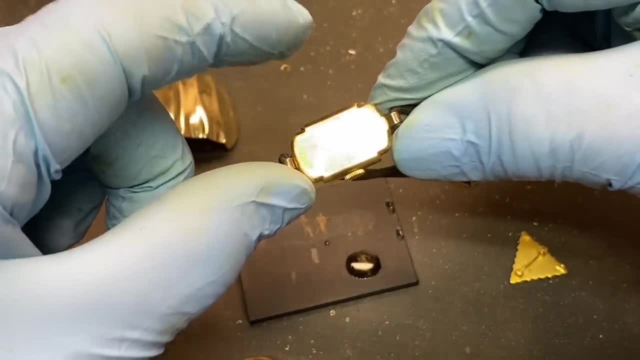 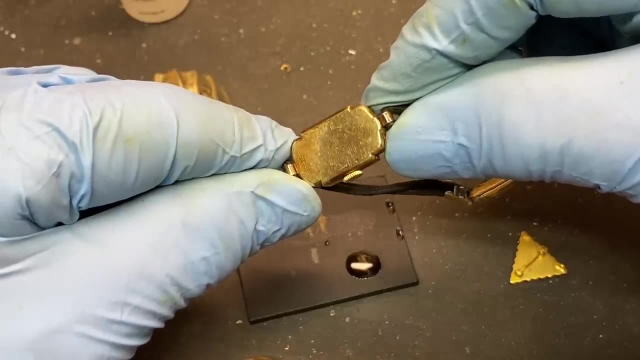 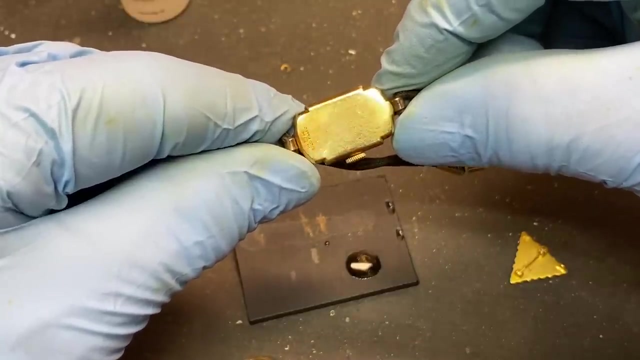 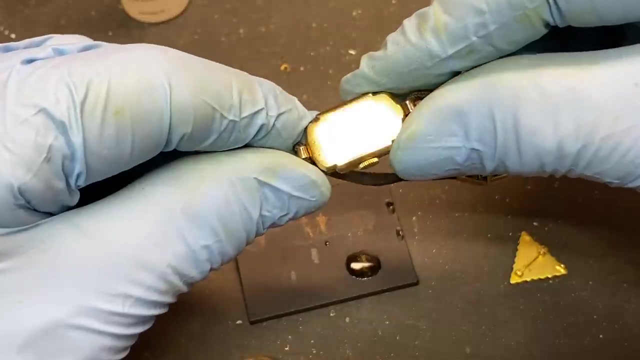 then you might mistakenly throw this piece in with your carrot scrap and that would skew your numbers for your in-quartation. When you calculated how much silver to add or copper to add to do the in-quartation, the gold content would go way low, too low, because you got brass under here. 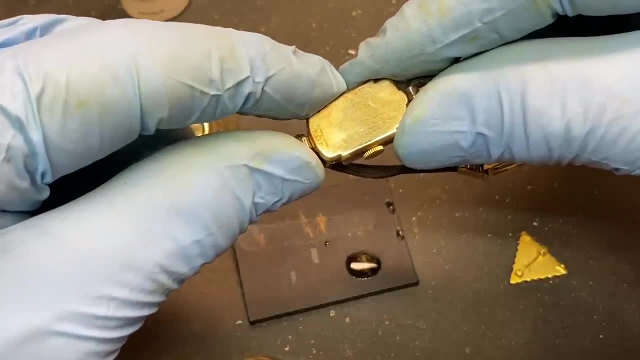 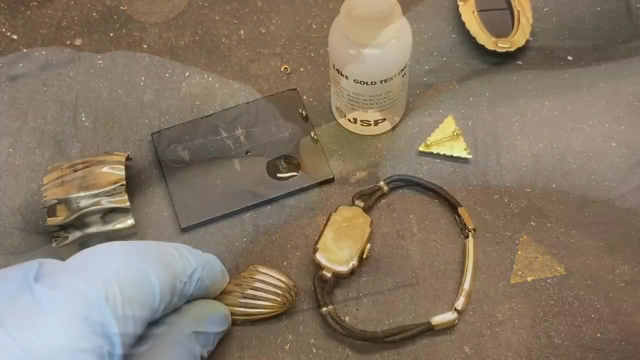 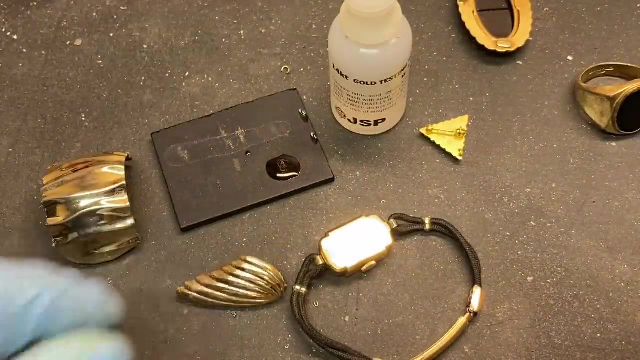 If you threw this in thinking it was gold, carrot gold, solid carrot gold, and then you'd end up with problems When you did the nitric boils. All right, what I have here is a piece of gold-plated material. If you notice, it will stick to my magnet. 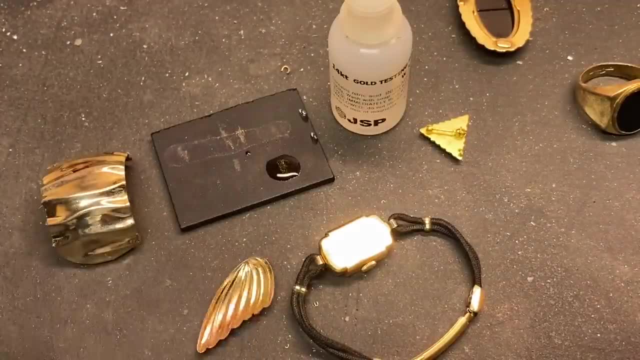 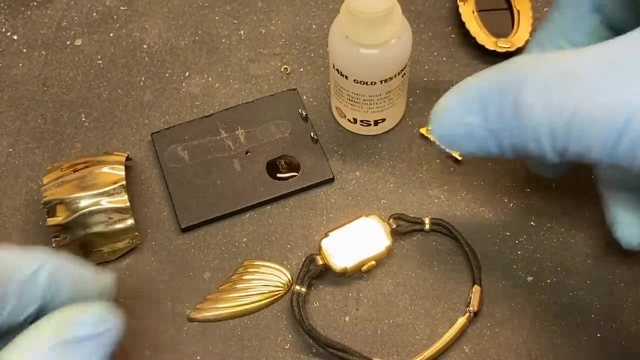 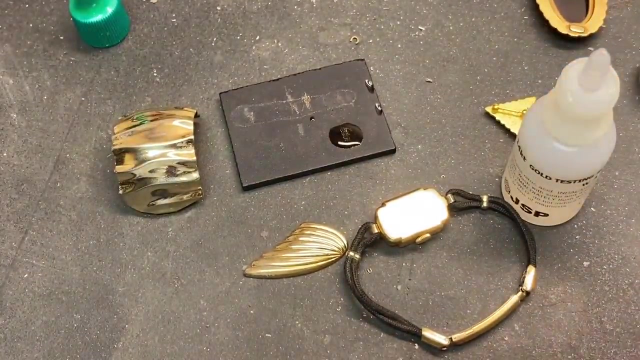 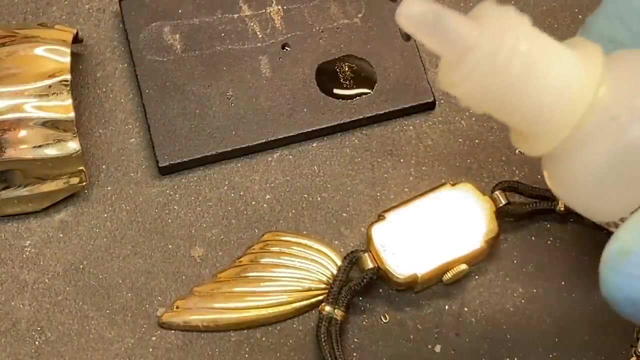 See that Normally carrot gold stuff doesn't do that. So what I'm going to do here is to illustrate how gold-plated material reacts with this test acid. I'm going to put a drop of the acid right directly on the gold-plated piece. 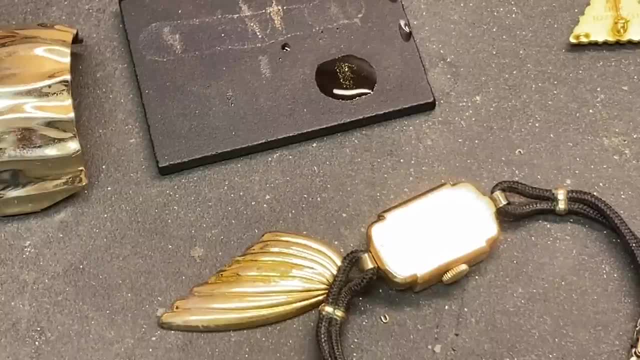 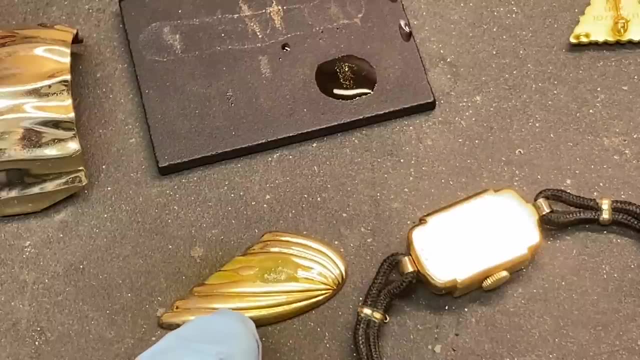 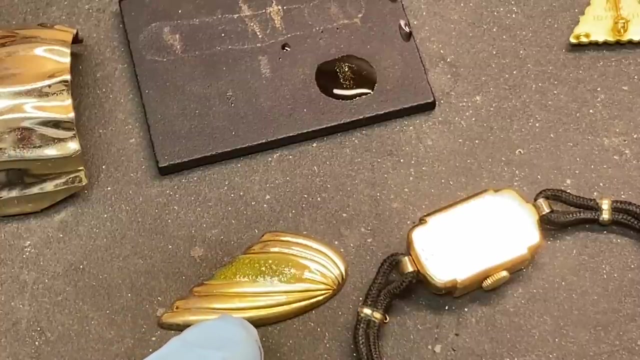 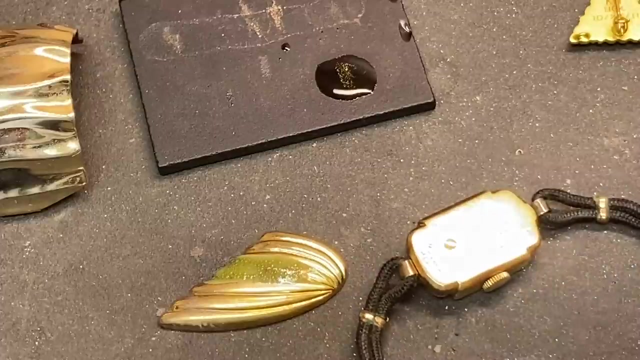 See how it immediately starts to bubble and boil. It turns green. That's because the acid is eating through the thin gold plating Almost immediately. That's how thin the gold is on there If you put the test acid on the gold-filled piece here. 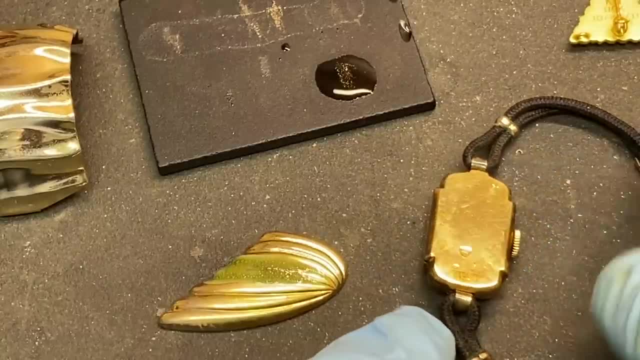 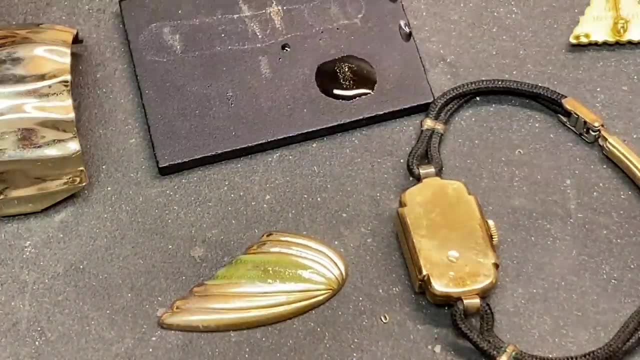 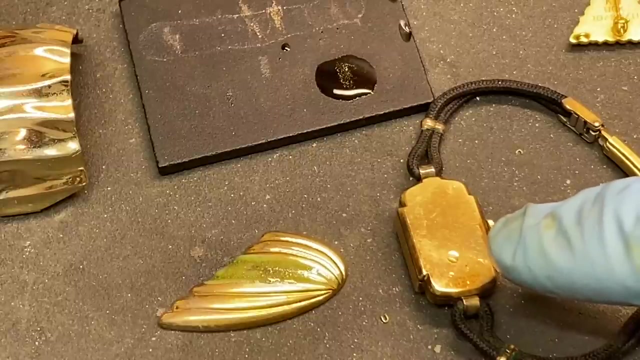 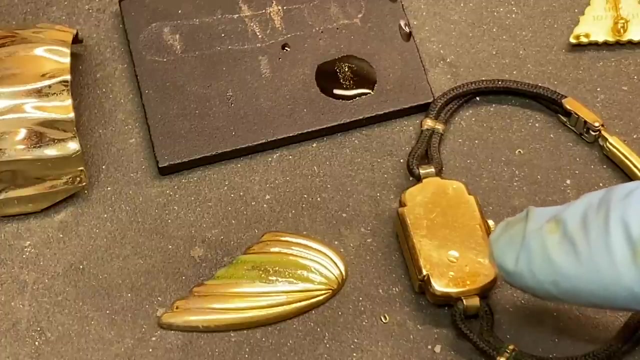 nothing will happen Because it's a thick coating of carrot gold over brass. It'll just sit there and it will not react. I could leave that on there all day and wipe this off And it would not get through that thick coating of 14K gold over that brass. 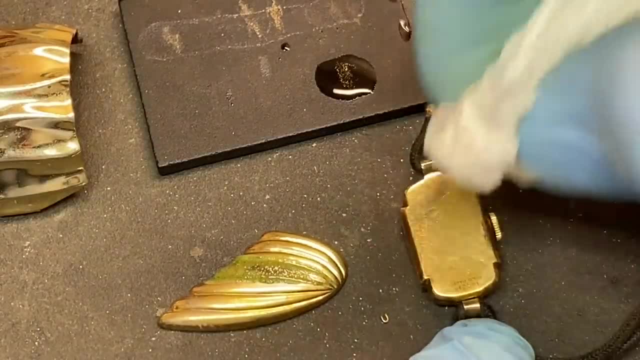 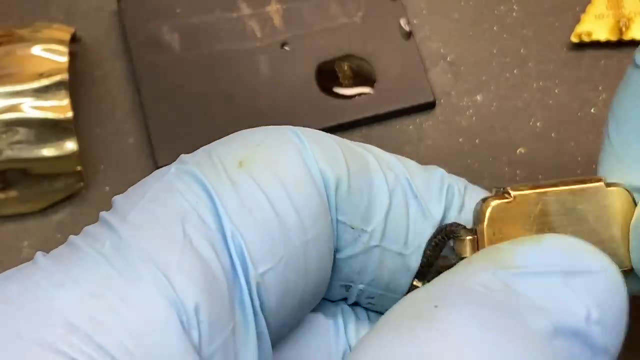 All right, I'm going to wipe this off. It's been sitting on there for over a minute. As you can see, it didn't react at all. Now, what I'm going to do is file a little bit of the metal off here. 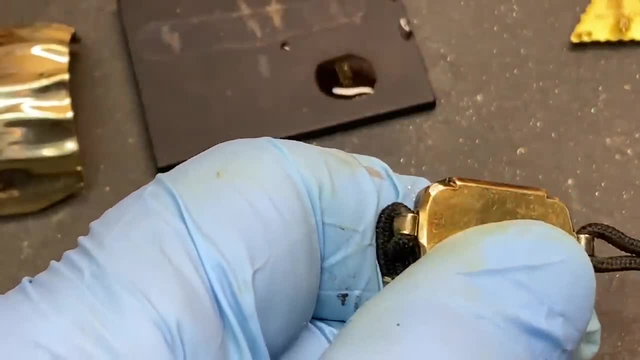 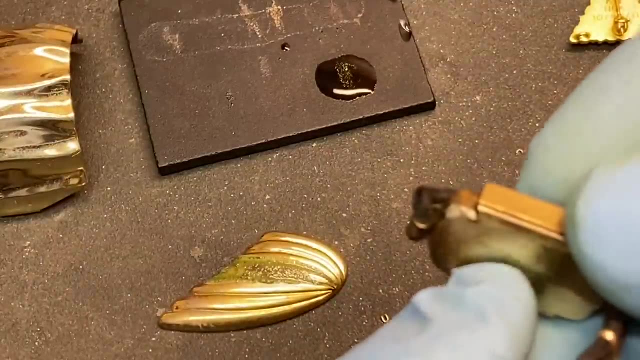 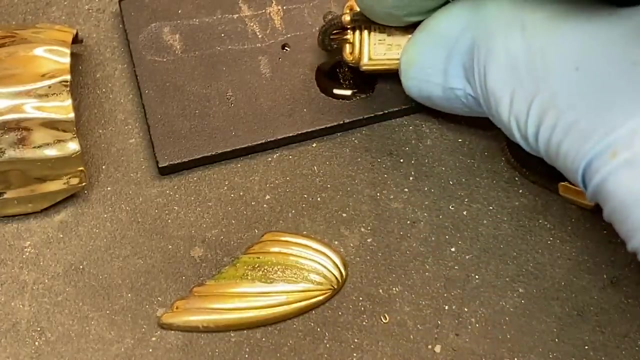 to expose the base metal under the carrot gold. And now what we'll do is dip this. Let's see where are we at on the camera. I'm going to dip that place that I just filed right there in this acid on our stone. 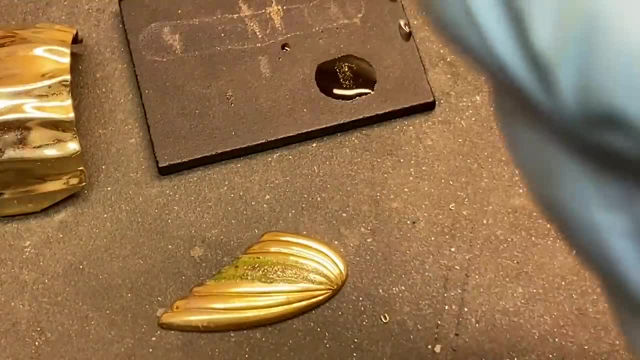 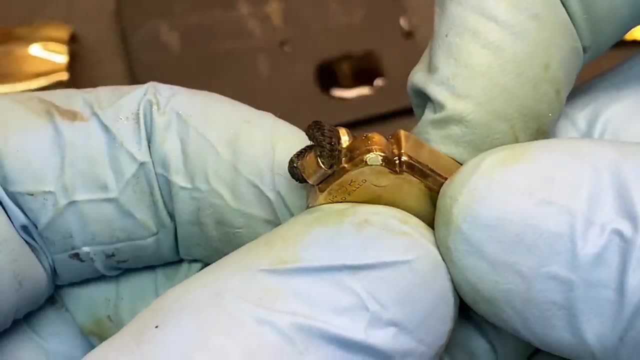 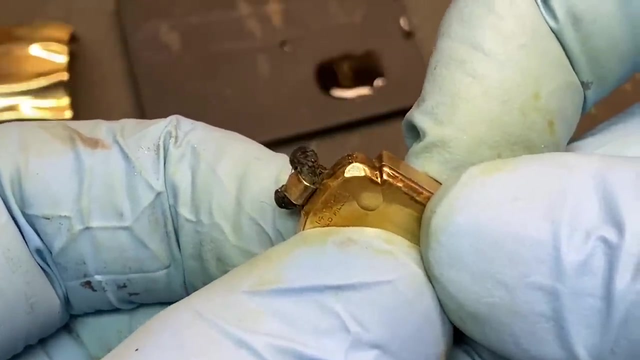 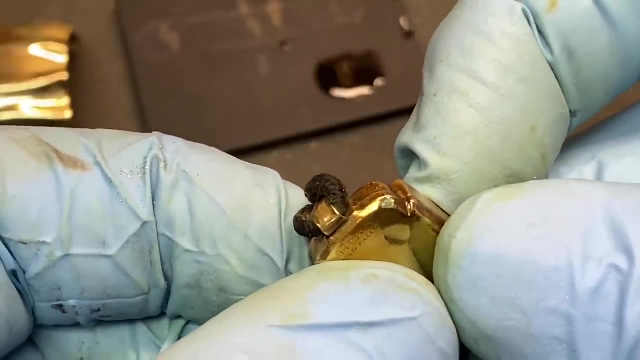 If I can do it without getting it all over the All. right, there we go Now. if you look, you'll see the acid immediately attacks the base metal underneath the brass, And there a distinct border becomes visible between the gold. 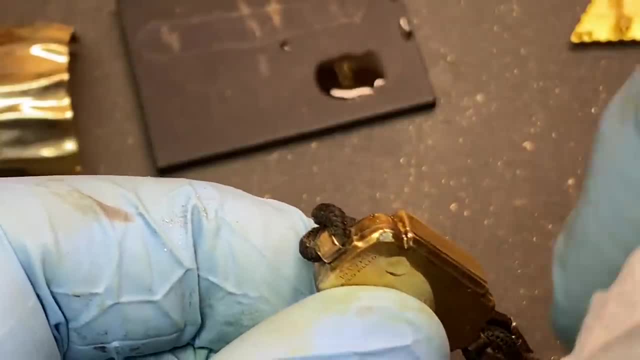 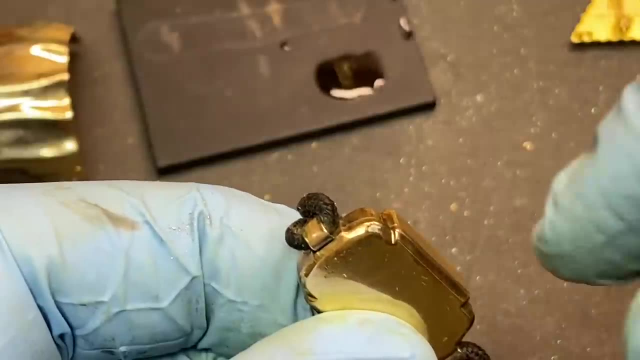 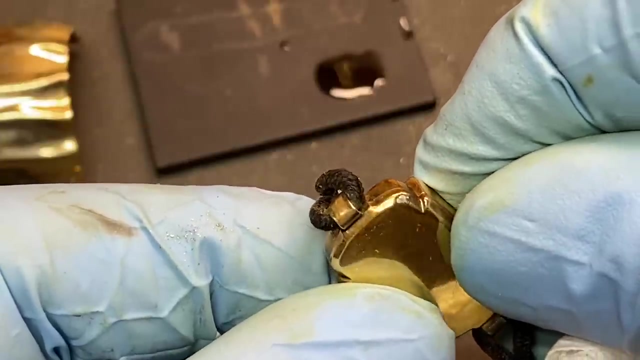 the thick plating of carrot gold over the brass. See it there. It's a very well-defined border. Let me wipe this off Now. you can see it real good. See the brass underneath And you got a thick coating of gold. 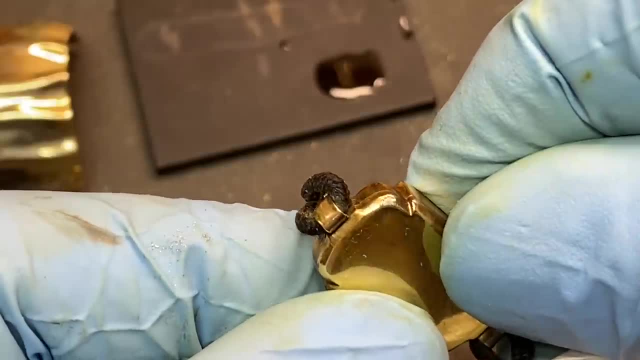 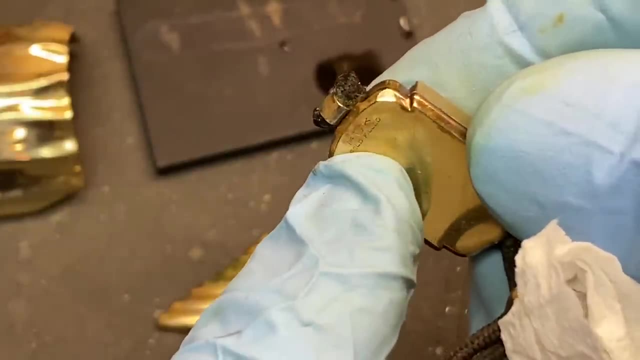 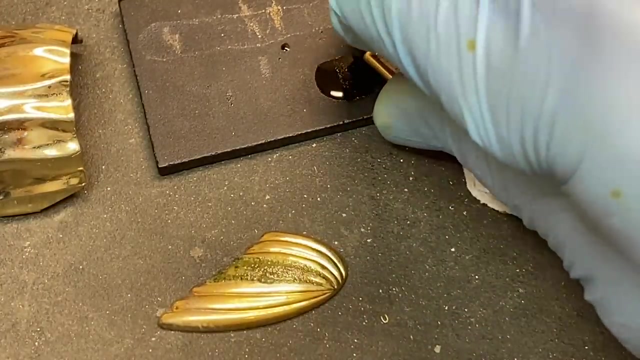 That's how thick it is. You can actually see it there And that's how we test for gold-filled material If it's not marked, like this one is, and we just file a little bit off and then dip the file mark into our acid.